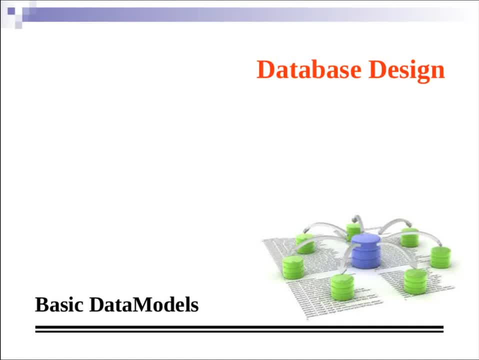 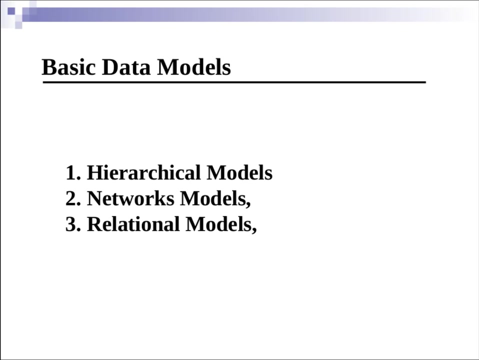 Hello, good morning everyone. On this lesson I will describe about database, basic data models, This presentation for introduction to learn the database before go to deeper lessons of database. On basic data model, there's three models. there are hierarchical models, networks models and relational models. 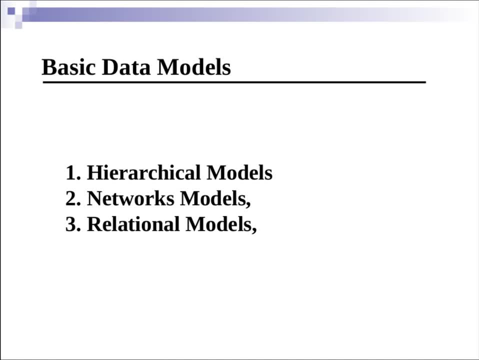 Hierarchical models, data is organized into a tree-like structure. This structure is simple but inflexible because the relationship is confined to a one-to-many relationship. The network model conceived as a flexible way of representing objects and their relationships, Each record to have multiple parent and child records. In the relational model, all data is represented in terms of tuples, grouped into relations. 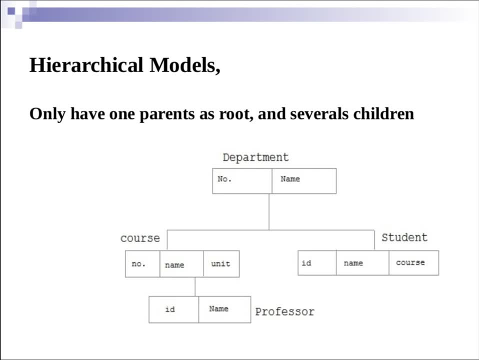 The hierarchical model structure was developed by IBM in the 1960s and used in early mainframe DBMS. Currently, hierarchical model are still widely used, especially in applications that require very high performance and availability, such as banking. 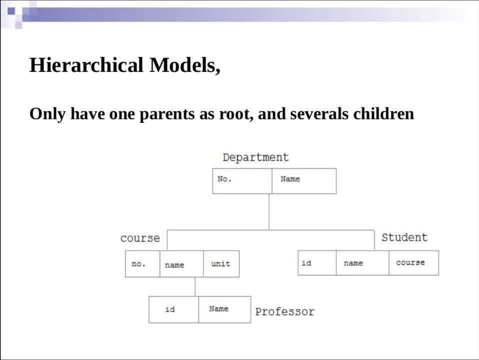 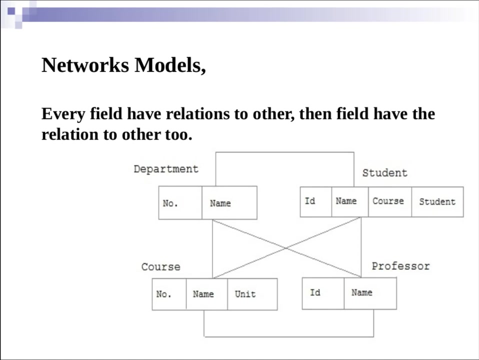 And telecommunications Hierarchical models only have one parent as root and several as children. Let's check the image below: The department tables become parents of course tables and student tables, And course tables become parents of lecturer tables. The network models. original inventor was Charles Bachmann and it was developed into a standard specification published in 1969,. 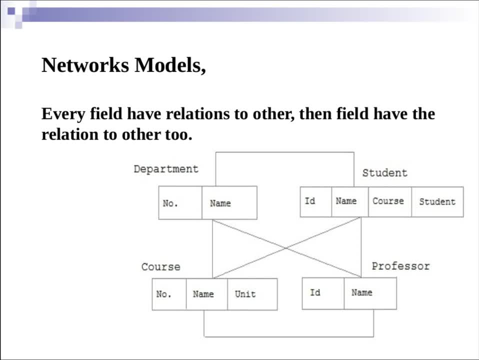 by the Texas Institute of ski and newspaper web. Shall I go back real quick? the Conference on Data Systems Languages Consortium. Every field have relations to other. On the display department, tables have a relation to student table, course table and lecturer table. 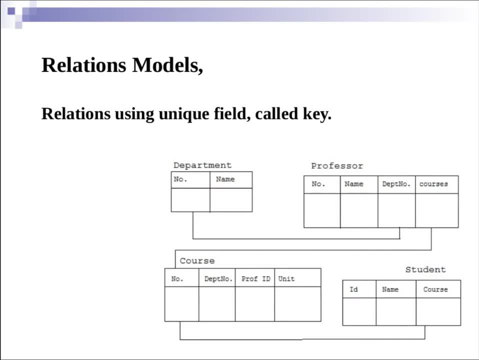 Relational model, first formulated and proposed in 1969, by Edgar F Codd. A database organized in relational model is called relational database On relational model. each relations using unique field called key To connect the table to table on the display. 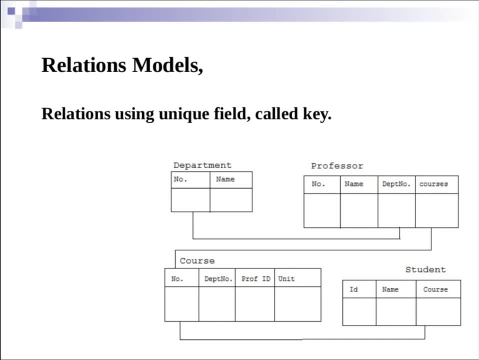 lecturer table have foreign key to store department ID and lecturer table have foreign key to store course ID. So lecturer table have two relations with department table and course table. Most relational database use the SQL SQL Data Definition and Query Language. 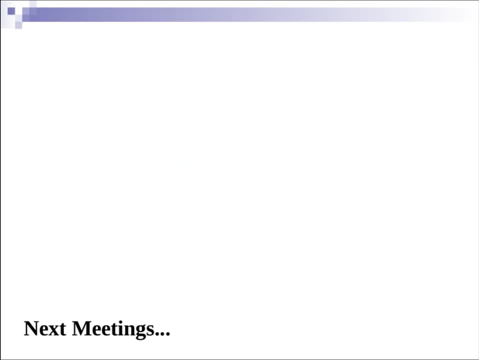 These systems implement the relational model. That's all the lesson about three basic data models. See you at next lesson. Thank you. 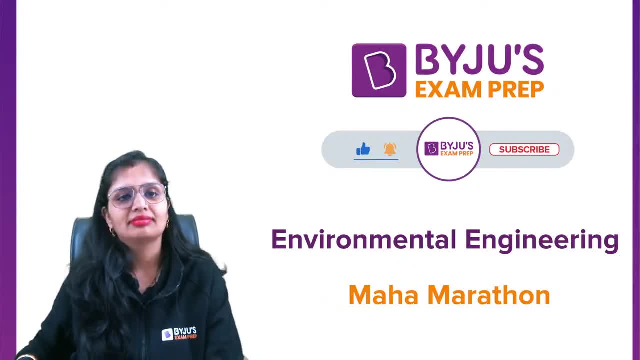 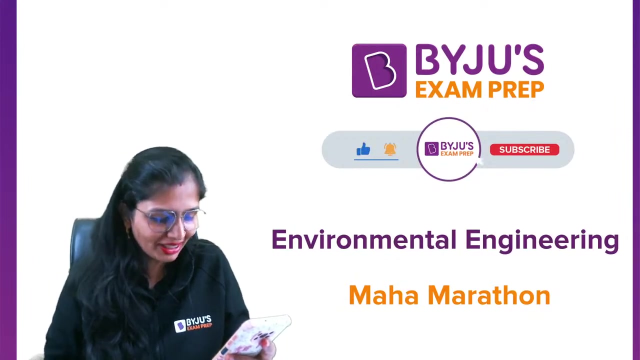 Hello everyone, welcome to Baiju's exam prep. Hope you guys are fine. So, guys, good morning everyone. Good morning Ready. Oh my god, I'm good, Arun, I'm good. Good morning Prince Arun, Ale Kakash, Padma Banot, everybody. good morning, Good morning everybody. So are. 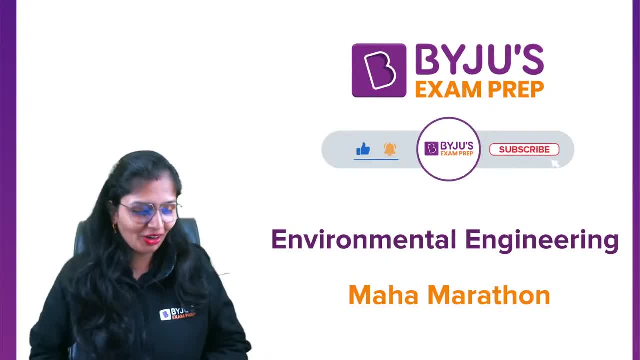 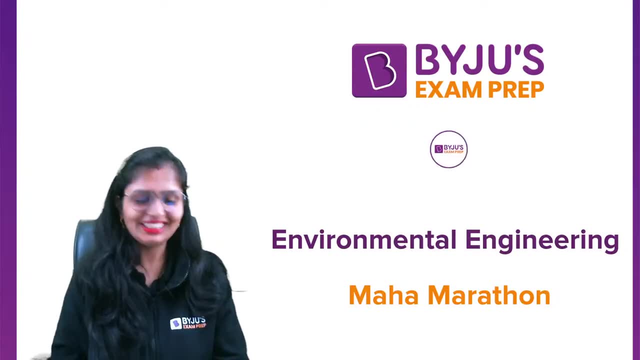 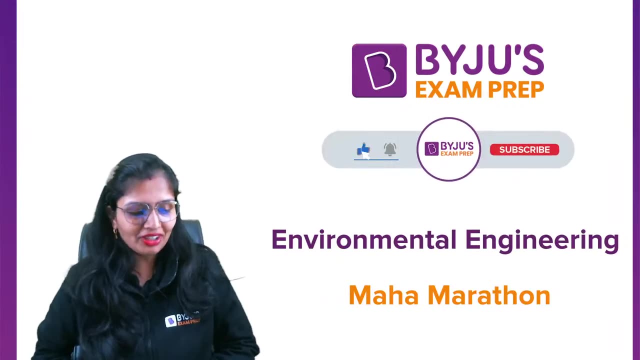 you guys excited Because today we'll be having a long day, and that too, by me only. I'll be the only one who will be taking the session. Good morning, good morning. So let's come on, guys, join fast. Good morning Vipul, good morning everyone. So had your breakfast, Had. 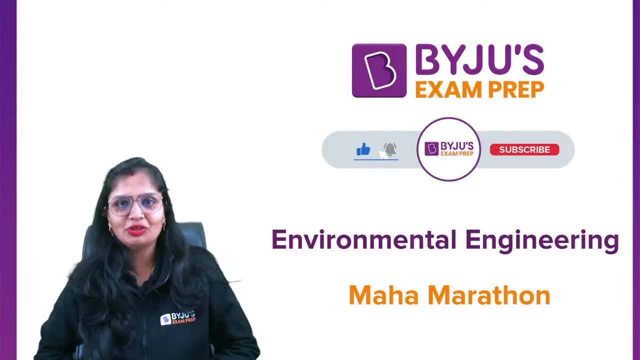 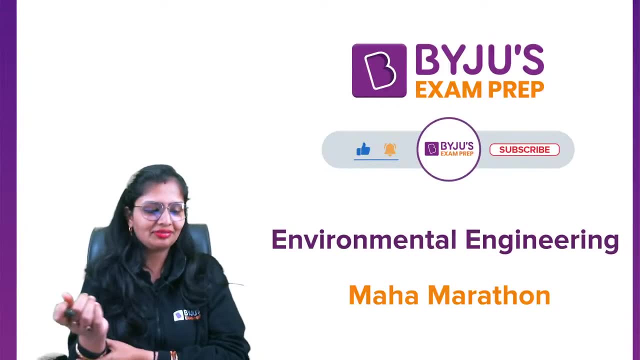 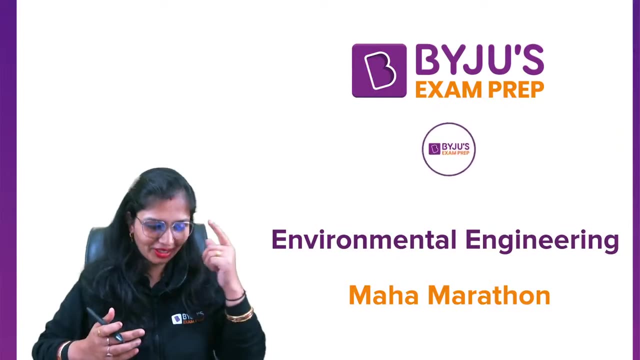 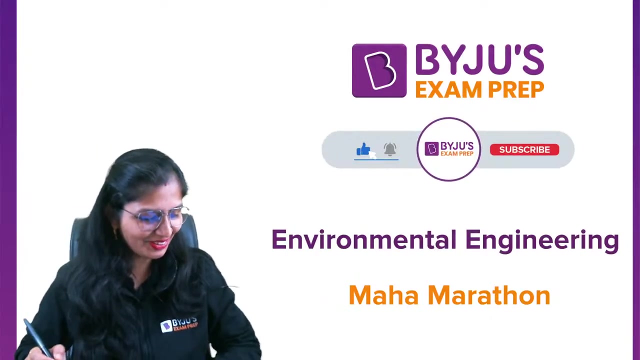 your breakfast. I told you to have your breakfast and come So that you don't feel hungry. Good morning, Good morning. Good morning, Pankaj. Okay, good, Good morning. At least girls listen to me. What about boys? Oh, boys also listen, Great. 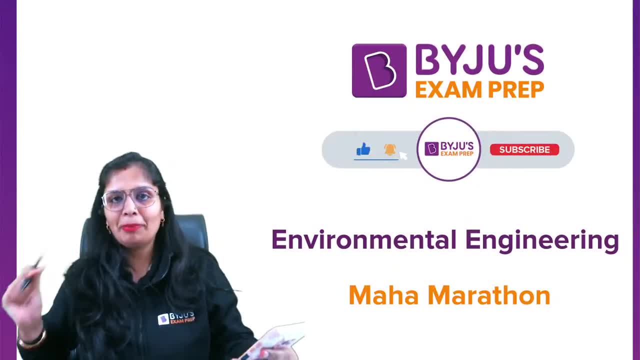 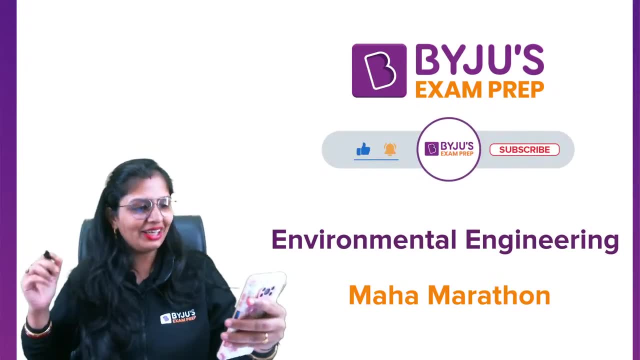 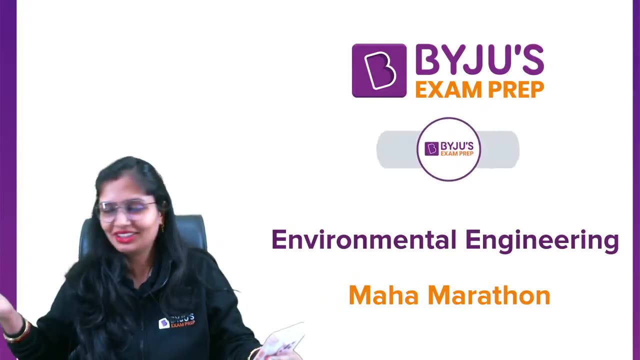 Okay, guys. So so you're ready with your pen, paper or copy and calculator Ready, Let's go. Good morning. Good morning, Rishabh. Oh, you woke up. I thought that you'll wake up late. Okay, See some people who answer quite frequently. I just have their names, like Rishabh Arun. 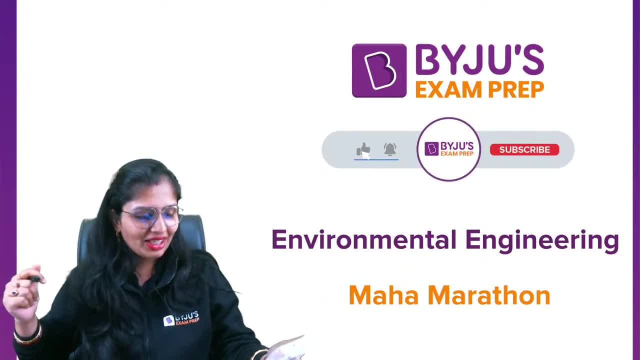 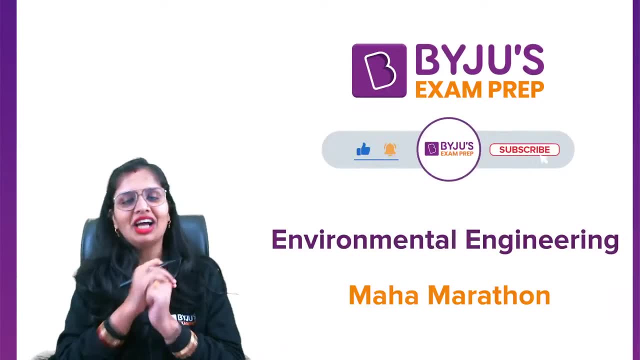